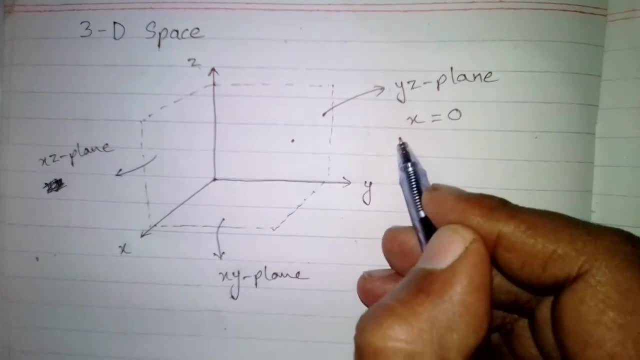 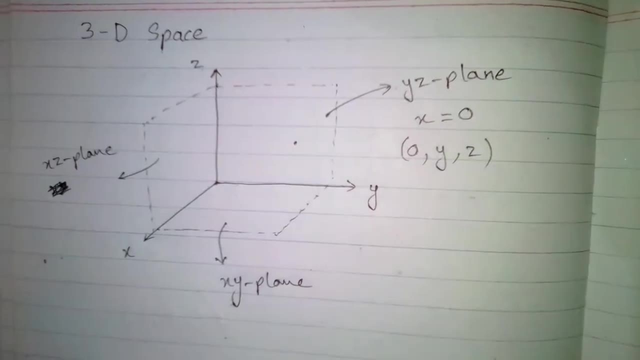 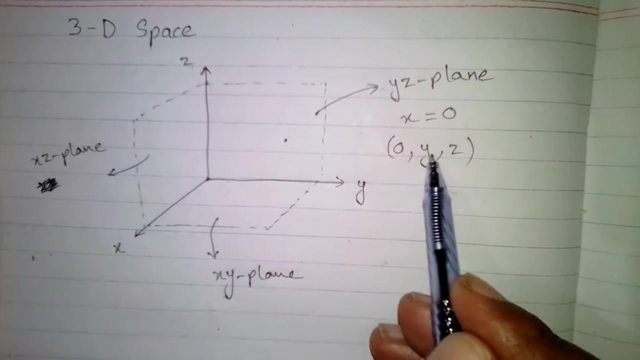 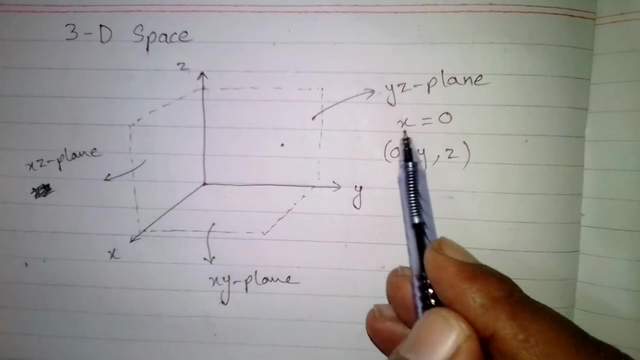 And we can write zero in place of X and YZ. So the point on the YZ plane is of the form zero. YZ because Y and Z has any value, zero and non-zero. but X has always equal to zero And this X is equal to zero is also zero. 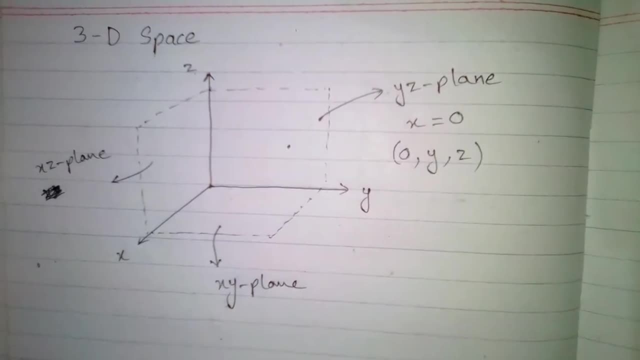 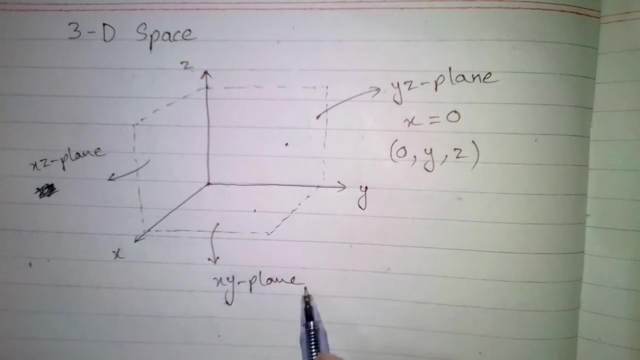 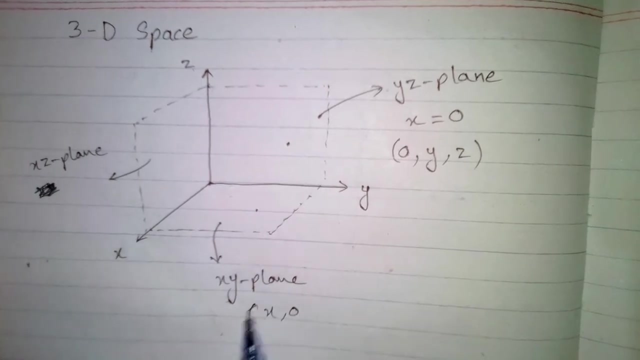 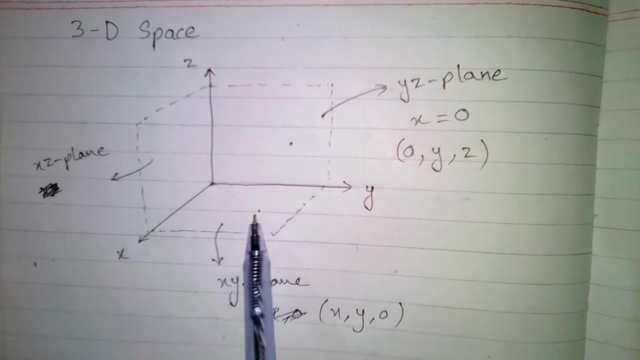 So the equation of the YZ plane, Similarly on the XY plane, if we take any point on XY plane, so this point is of the form X: 0, sorry, X Y 0, because the Z component on the XY plane is always zero. 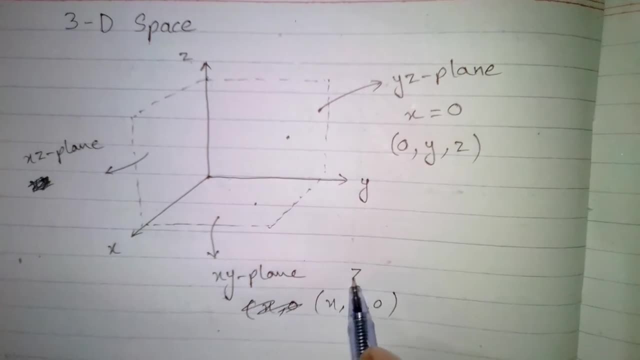 And the equation of the YZ plane is of the form zero. So the equation of the YZ plane is of the form zero. So the equation of the YZ plane is of the form zero. So the equation of the XY plane is: Z is equal to zero. 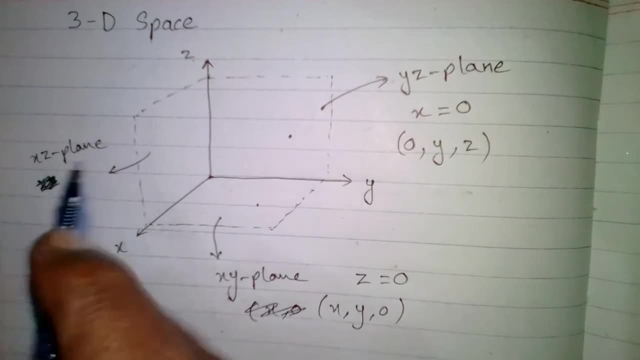 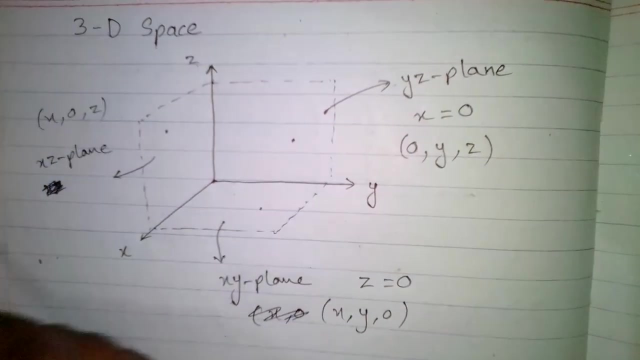 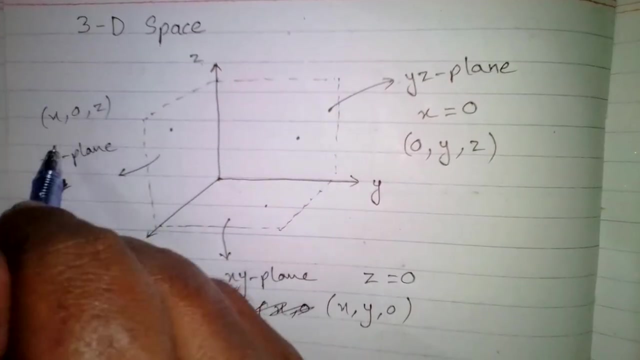 Similarly on the XZ plane, if we take any point. so this point is of the form X, 0, Z and the value of Y on the XZ plane is always zero. So the equation of the XZ plane is: Y is equal to zero. 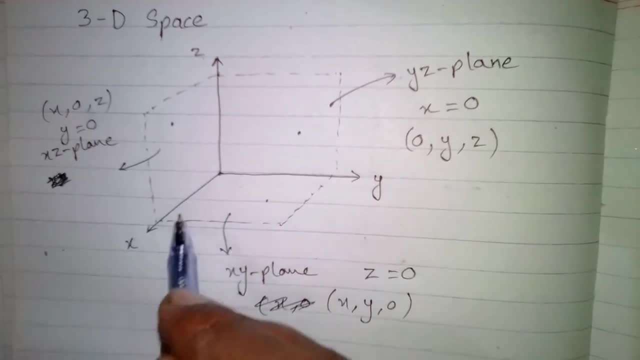 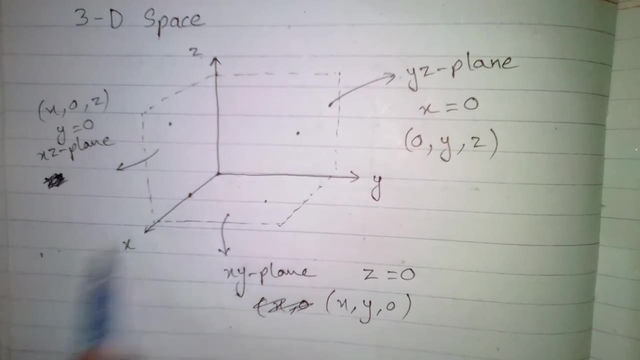 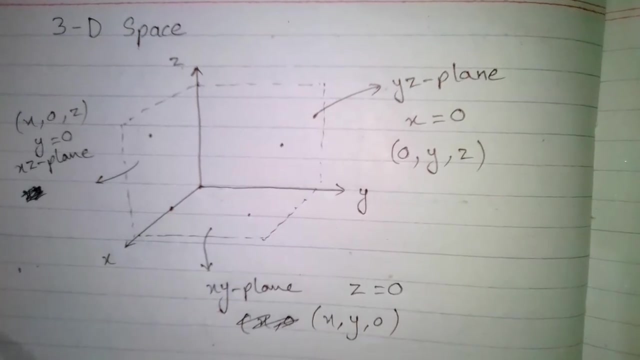 So the equation of the XZ plane is: Y is equal to zero. we take any point on the x-axis. so the point on the x-axis has x component may be equal to 0 or nonzero, but y and z component are always equal to 0. so the 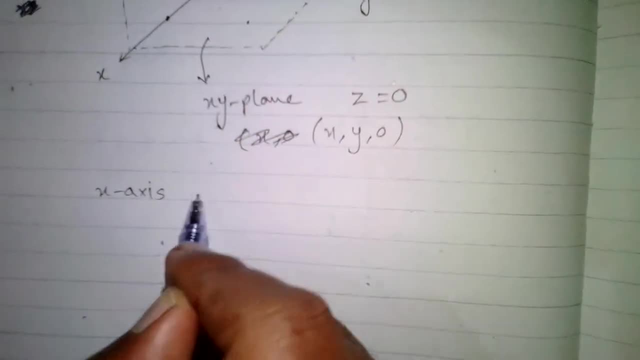 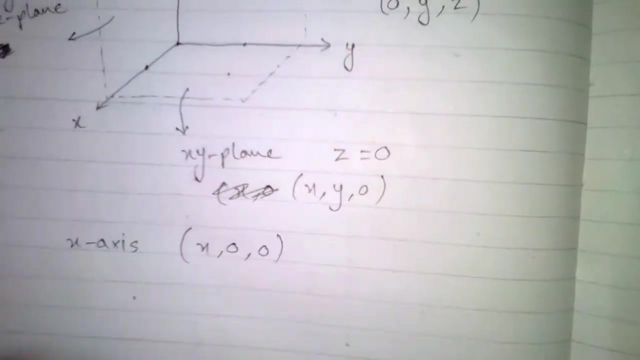 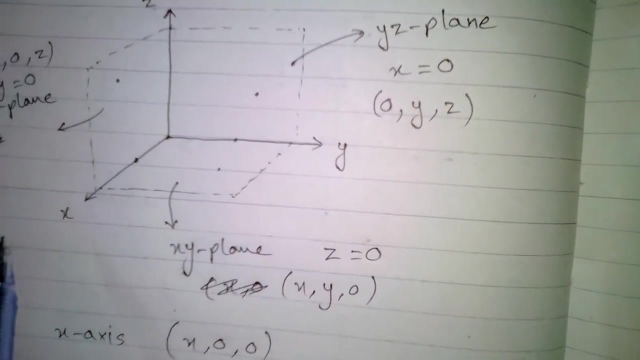 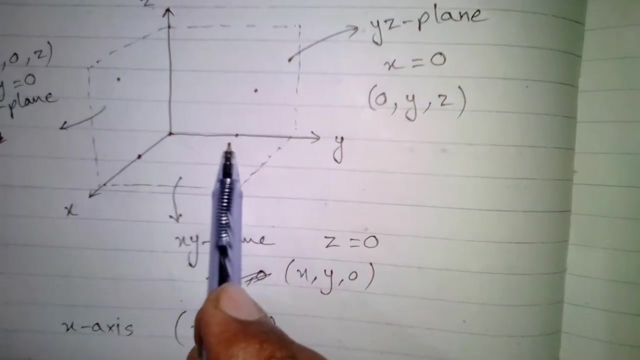 point on the x-axis is of the form x comma 0, comma 0. now if we take point on the y-axis, so this point has y component equal to 0 or may be not equal to 0, nor nonzero value, but the x component and z component are always 0. so on y-axis the 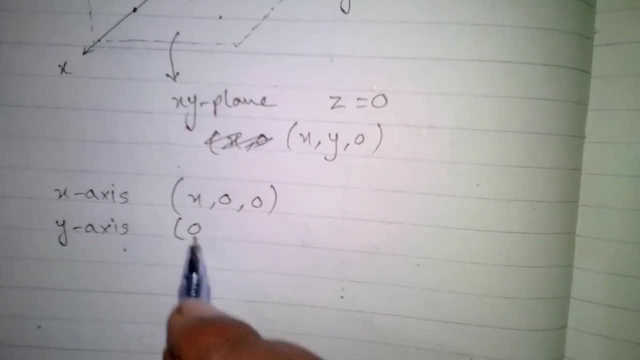 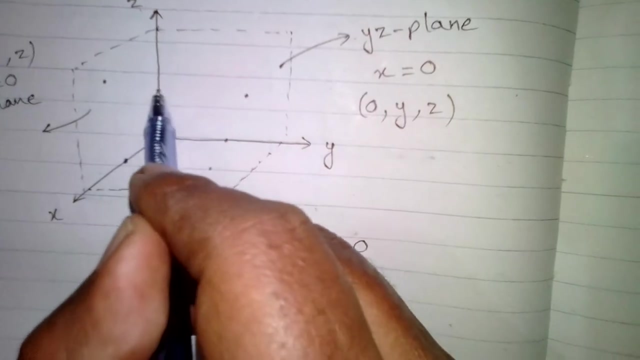 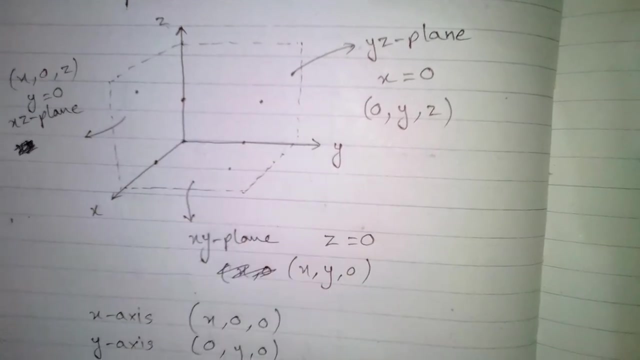 points are always equal to 0. so the point on the x-axis is of the form x comma 0, is of the form 0 comma y comma 0. similarly, on the z-axis, the value of z may be 0 or nonzero, but the value of x and y will always be 0. so the point on 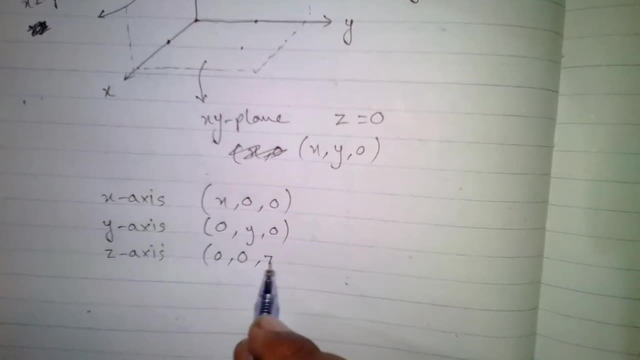 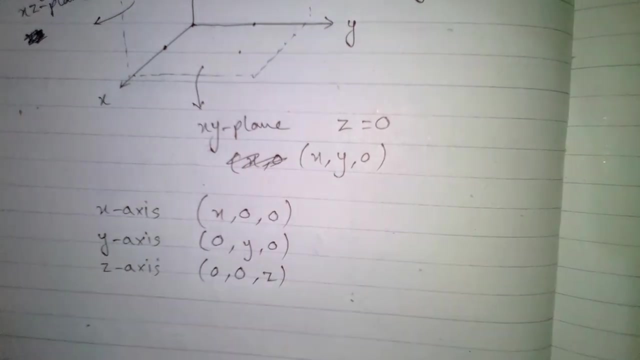 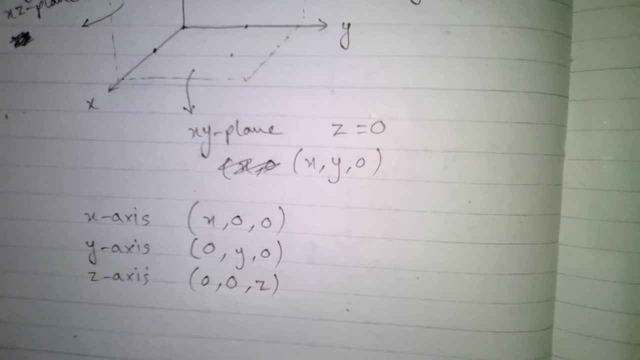 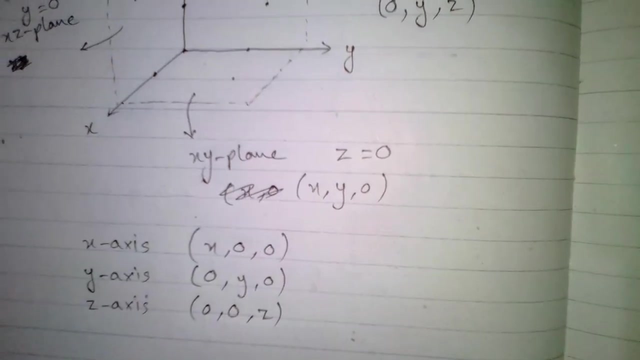 the x-axis is of the form 0 comma 0 comma z. so these are the point in 3 dimensional space and we have seen that. what is the form of the point on x-axis, y-axis and z-axis and what are the forms on the xy plane, yz plane and zx plane? 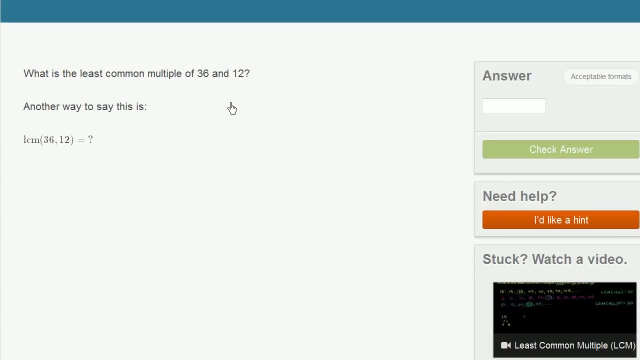 What is the least common multiple of 36 and 12?? So another way to say this is LCM, in parentheses: 36 and 12.. And this is literally saying what's the least common multiple of 36 and 12?? Well, this one might pop out at you. 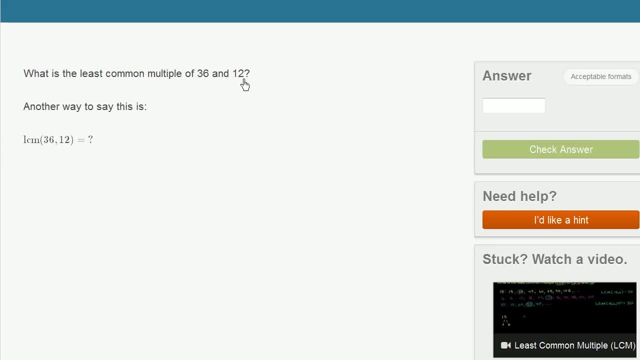 because 36 itself is a multiple of 12.. And 36 is also a multiple of 36.. It's 1 times 36.. So the smallest number, that is both a multiple of 36 and 12, because 36 is a multiple of 12, is: 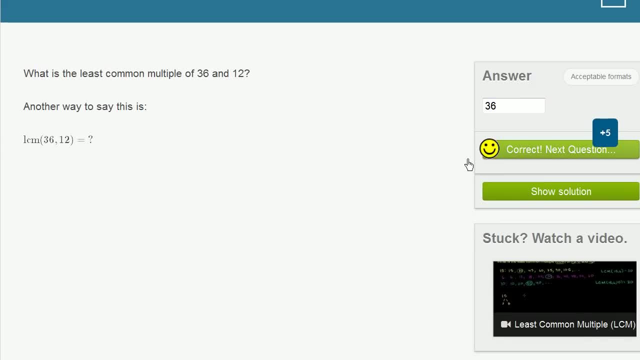 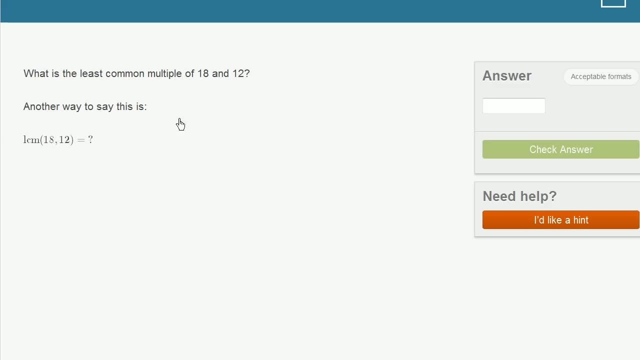 actually 36.. There we go. Let's do a couple more of these. That one was too easy. What is the least common multiple of 18 and 12?? And they just state this with a different notation: What's the least common multiple of 18 and 12? 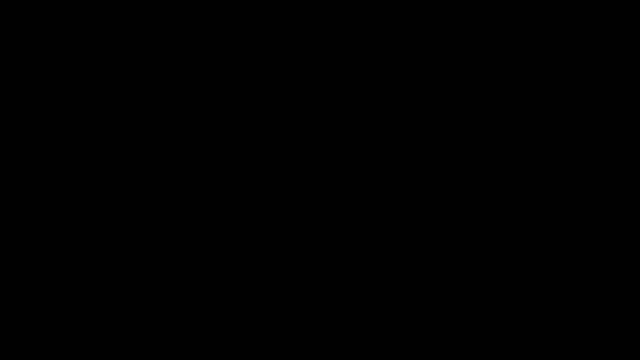 is equal to question mark. So let's think about this a little bit. So there's a couple of ways you can think about. So let's just write down our numbers that we care about. We care about 18 and we care about 12.. 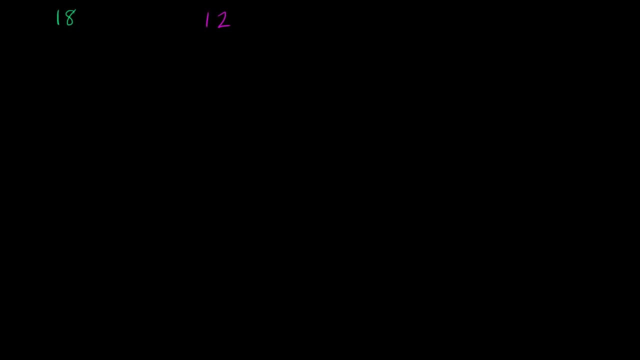 So there's two ways that we can approach this. One is the prime factorization approach. We can take the prime factorization of both of these numbers and then construct the smallest number whose prime factorization has all of the ingredients of both of these numbers.